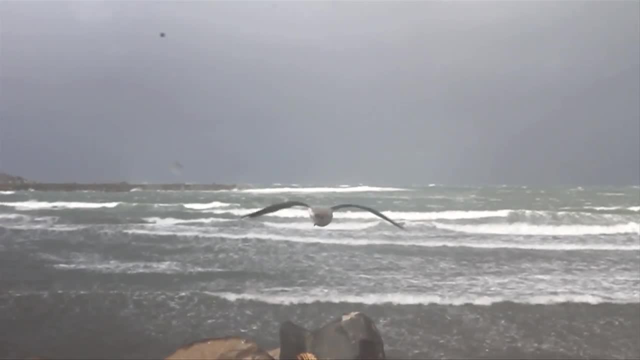 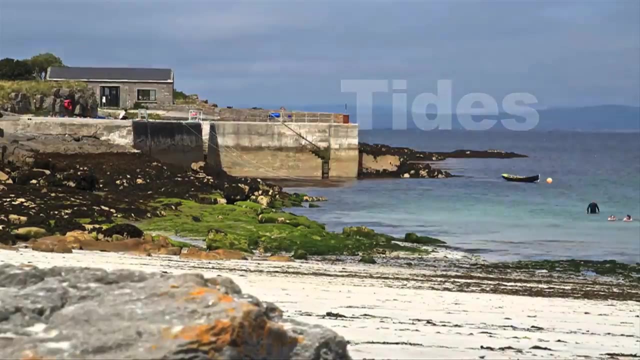 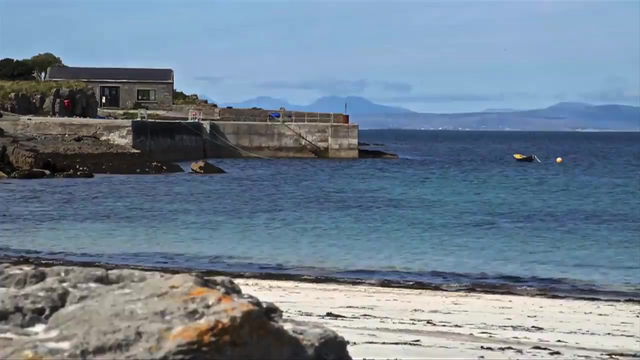 If the wind comes from the water towards the beach, that's onshore, and the waves are going to look like this. Tides influence waves by changing the depth of water at a surf spot. As tides change, the waves will break in a different place over different contours of the sea floor. Some surf 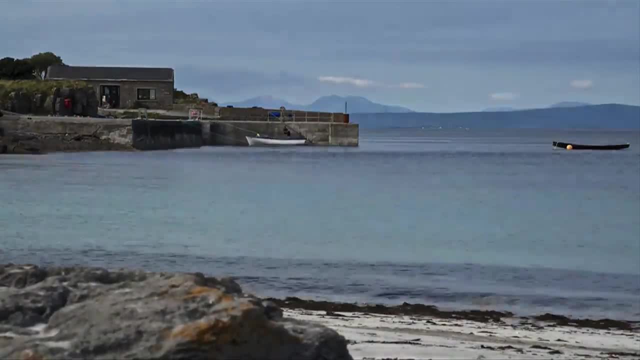 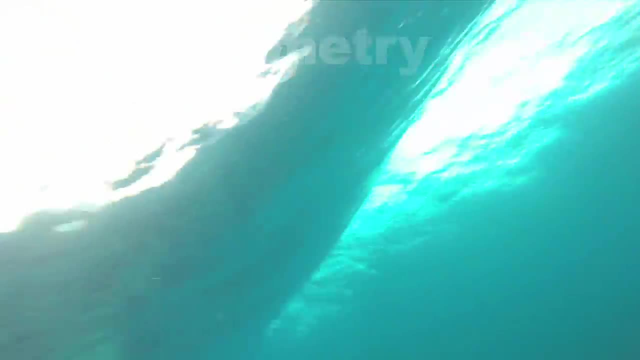 spots will only be good on a very specific tide, while others will have good waves on all tides. Finally, it's the shape of the rock or sand underneath the water, the sea floor. This is what waves their shape and is probably the most important. Now let's take a close. 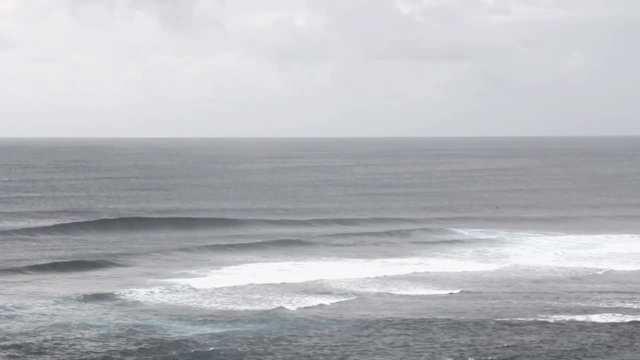 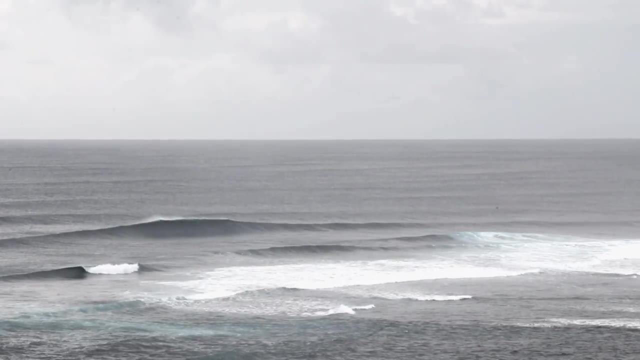 look at this surf break. The wind is good light offshore. The swell is about two meters coming from the southwest, with about a 13 second period. At this particular spot you can surf on most tides. Things are looking good. This is. 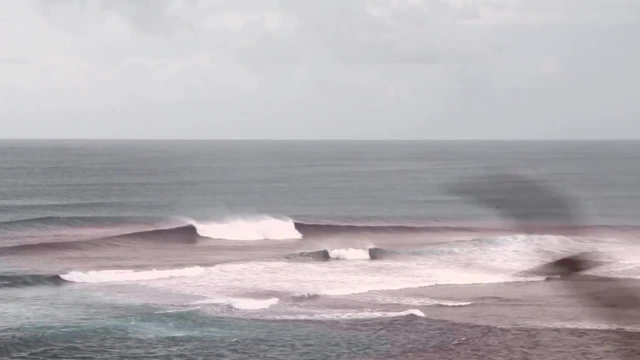 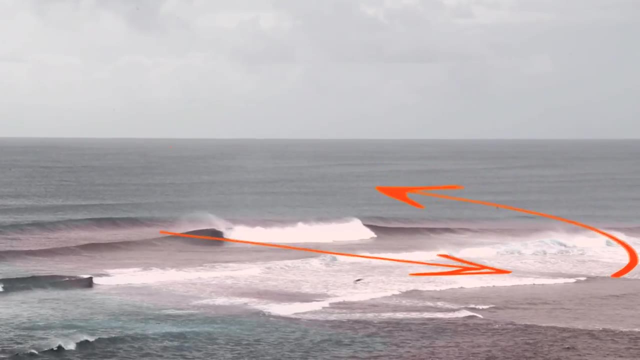 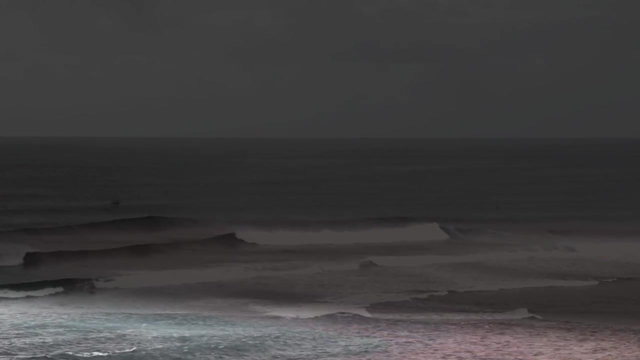 shallow water. We can tell because the waves are taller. here. they're being lifted up by the sea floor. underneath The water pushes in towards the beach where it's shallow. then it finds deep channels nearby, turns around and goes back out to sea. Look closely at the texture of the water here: it's rough and 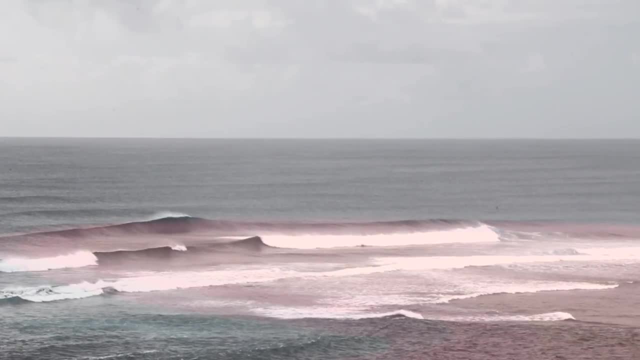 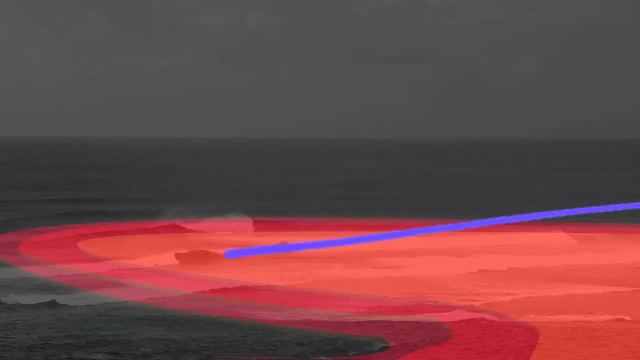 peaky. That's showing us two opposing flows of water. We want the swell line to run along the edge of a sandbank or reef, hitting shallow water, and an angle like this. This will make the wave peel. The opposite is a wave that arrives. 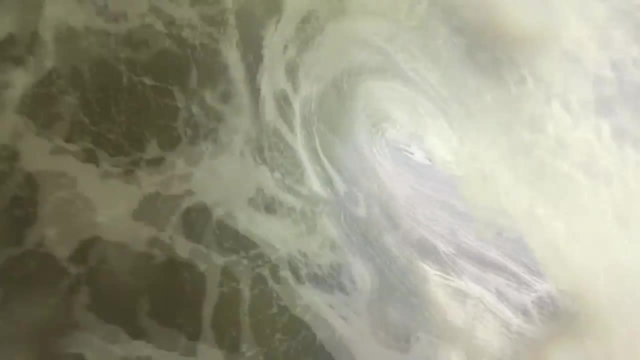 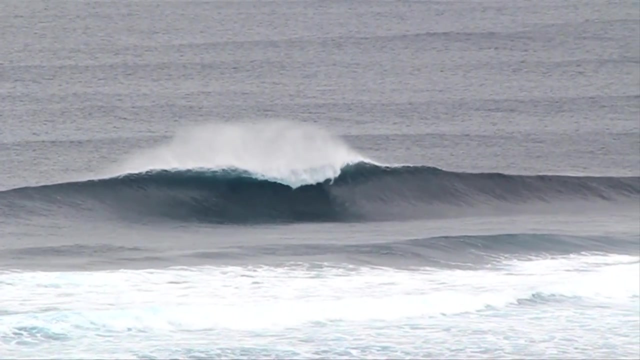 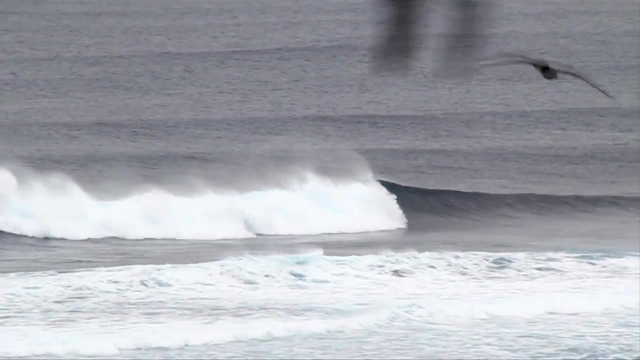 parallel to shallow water, a closeout. We can't surf closeouts. there's nowhere to go. As the wave peels, it's feeling out the sea floor. The bathymetry will decide the shape and power of the breaking wave above. If the sea floor has a steep angle, the wave will 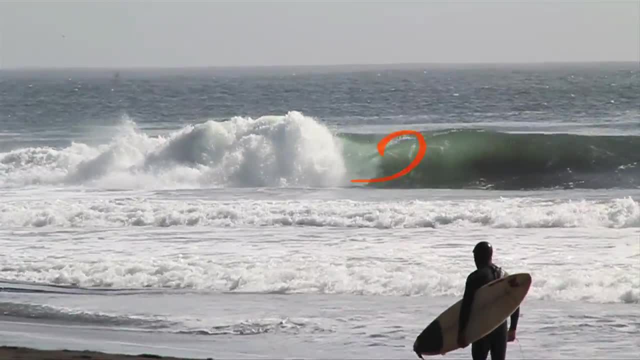 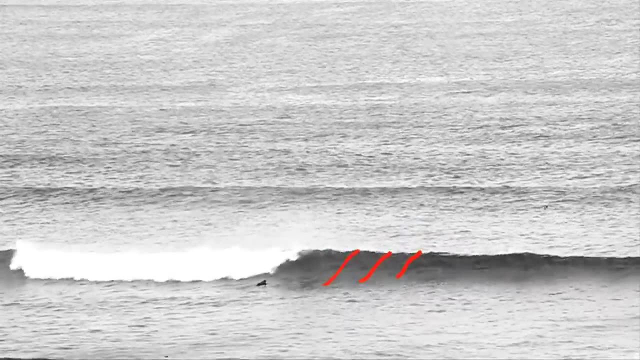 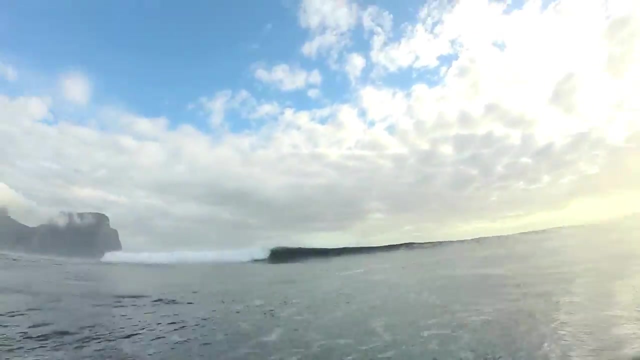 be powerful, characterized by a tubular shape. If the slope of the sea floor is flatter, the wave will be softer, more slopey and it will be breaking in deeper water. But waves can do both. Look at this wave as it travels through different sections of reef, As it 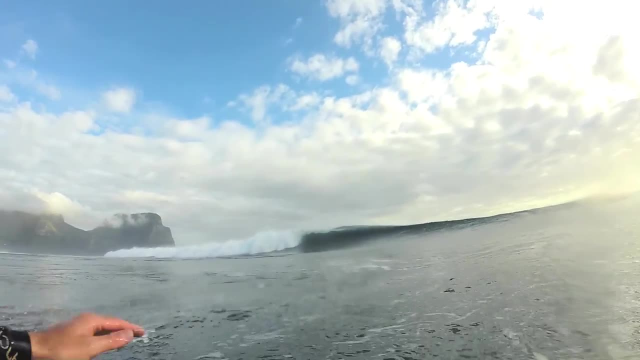 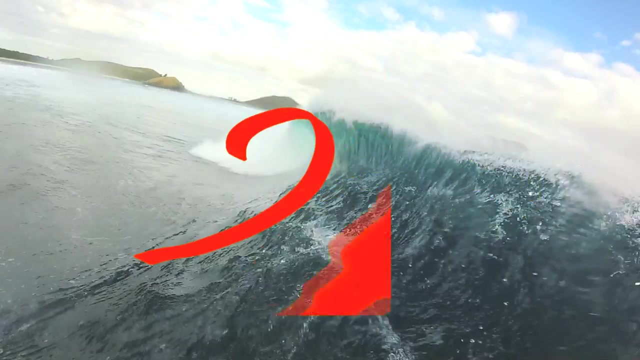 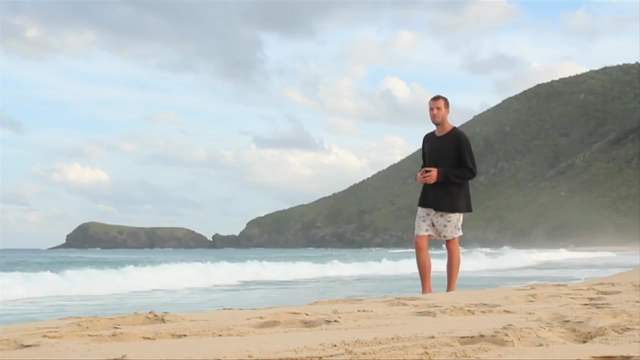 breaks, it's quite powerful, Then it goes a bit soft, Then it hits some shallow water and gets heavy again. The shapes and curves of the waves are subtle, but tell us exactly what is happening underneath the water And it's understanding these subtle curves and